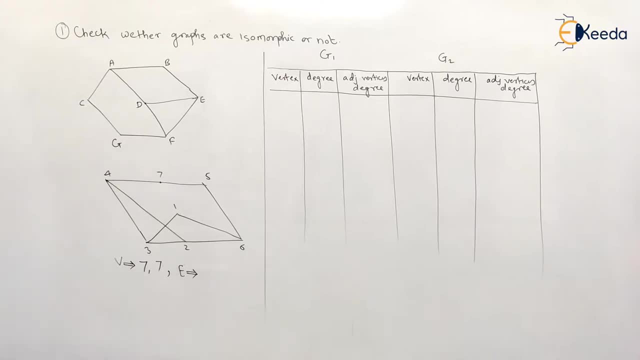 number one satisfied. Let me check how many edges are there In the problem? So, how many edges are there? Let us check. See one, two, three, four, five, six, seven, eight. So there are eight pages here. Let's talk about this. One, two, thee, four, five, six. 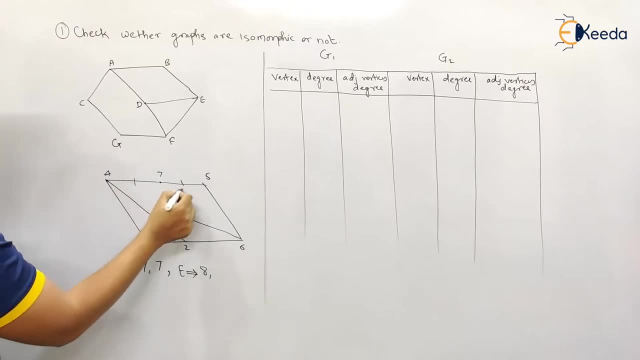 seven, eight, nine. Let me count again: one, two, three, four, five, six, seven, eight nine. So there are nine edges. Let me check again one, two, three, four, five, six, seven, eight, nine again. 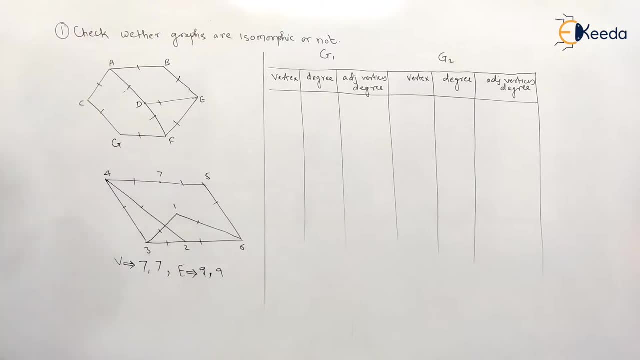 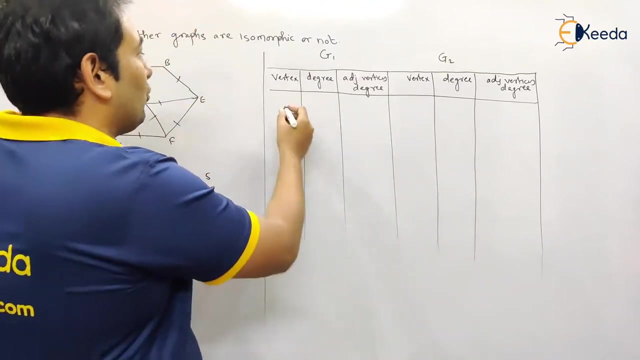 and 9. so condition satisfied: number of edges and number of vertices are same. point number three: they should have same degrees of vertices. so let me check for that for that purpose. let us do. let us make this table first. let us make this table first. vertex and degree. so how many vertices are? 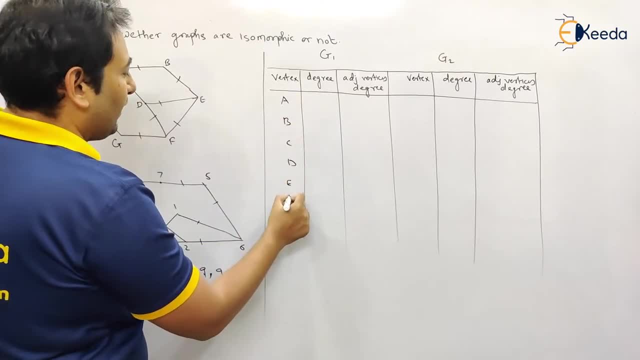 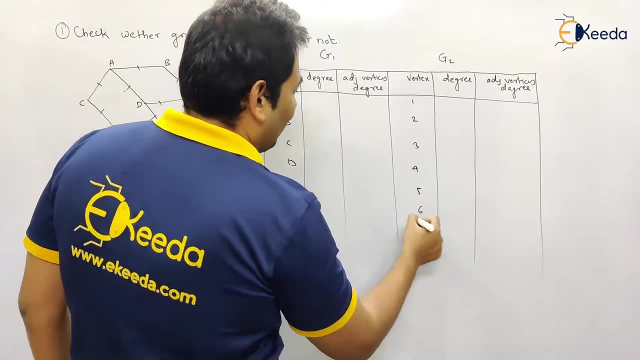 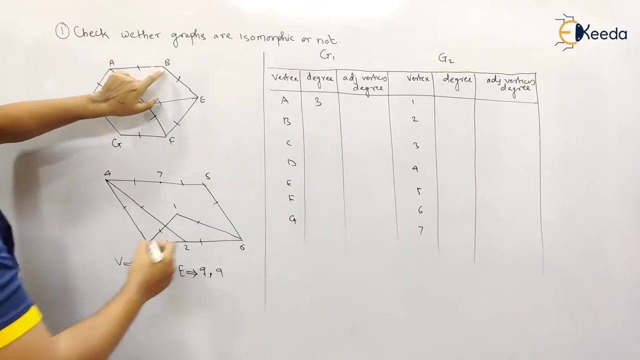 there in graph number one, a, b, c, d, e, f, g, and here we have one, two, three, four, five, six, seven. let us count the degrees. so a: a degree is three, b, b degree is two, c, c degree is again two, d, d degree is one, two, three, e degree is three, f, f degree is three and g degree is two. now let us check for. 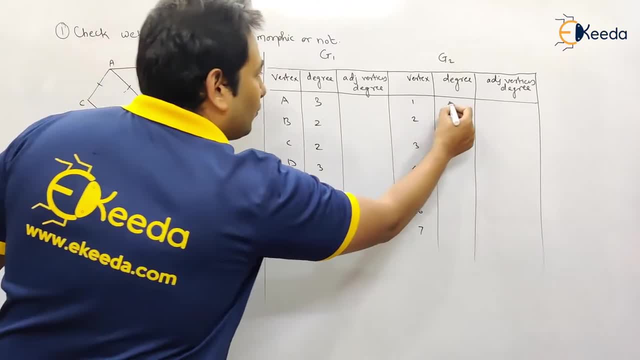 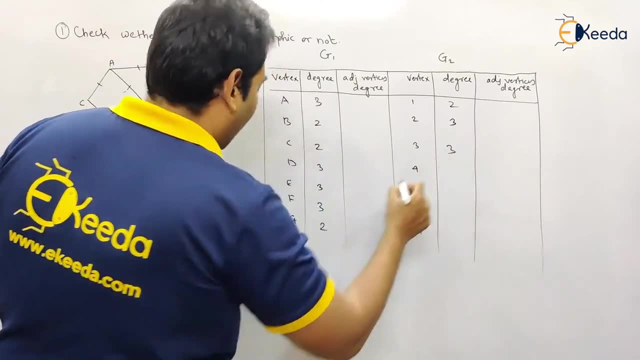 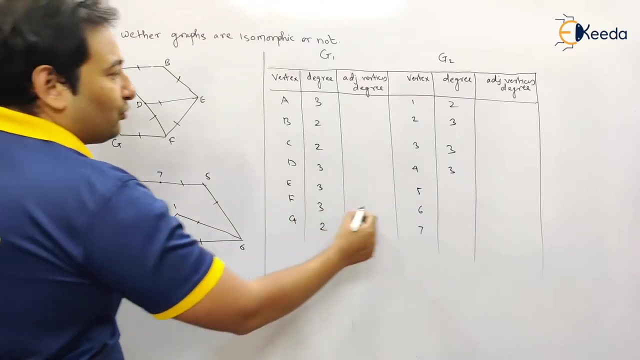 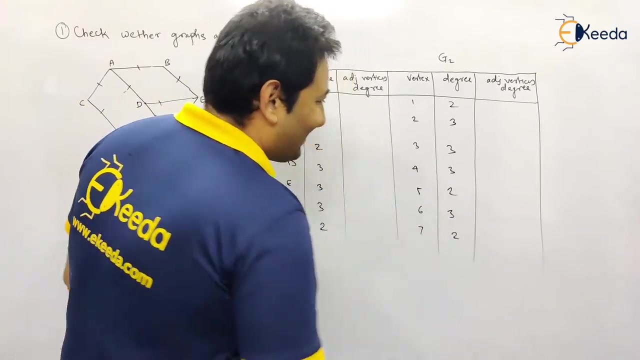 vertex one, two, three, four. this is in graph two. one degree is two, next two degree is three. three degree is again three, next four degree is again three. five degree five is two, six is three and seven is two. now let us check how many vertices with degree two. so there are three. 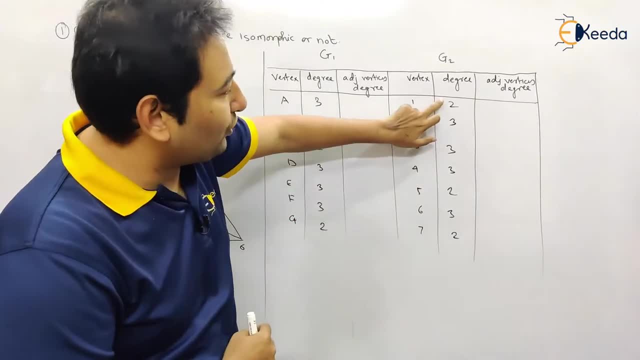 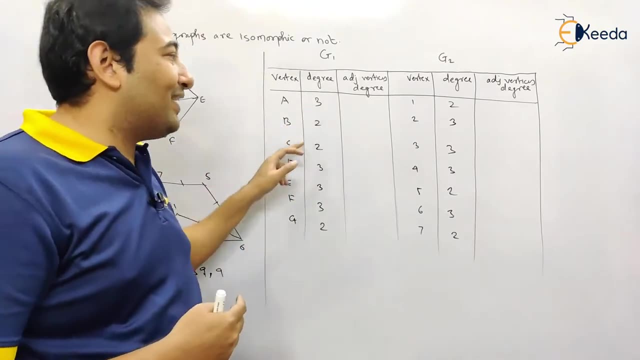 vertices with degree two. here also there are three vertices with degree two, fine. next there There are 1,, 2,, 3, 4.. There are 4 vertices with degree 3.. There are 4 vertices with degree 3.. That means point number 3 is satisfied. 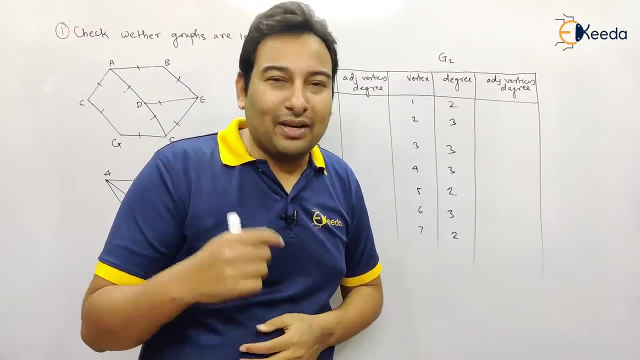 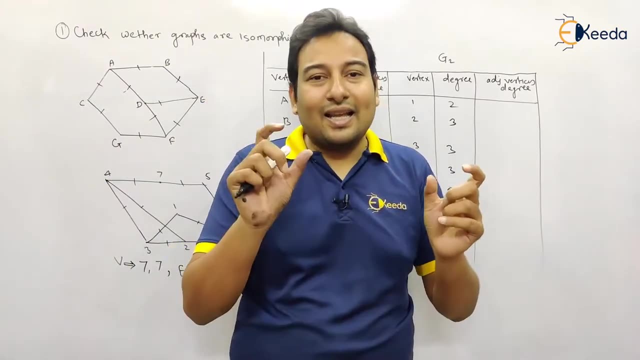 What next? Number 4.. For last point, we need to rename it. Remember the last problem, what we did, 1, A, 2, B. In that problem the renaming was very simple Because both the graphs were having vertex with degree 2.. 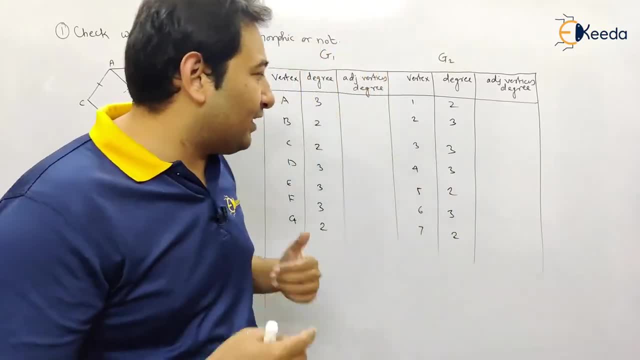 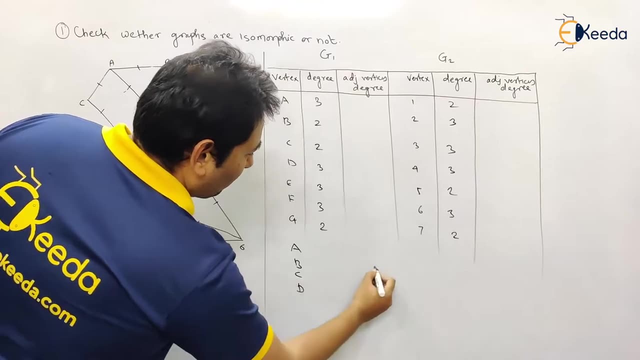 Each vertex with degree 2.. But here there is a difference. So while renaming it you should be careful. That means you cannot simply write it down. See, my aim is to rename it Simply. I cannot write it down as 1,, 2,, 3.. 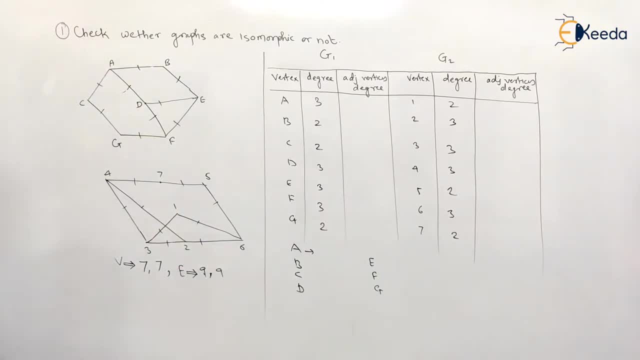 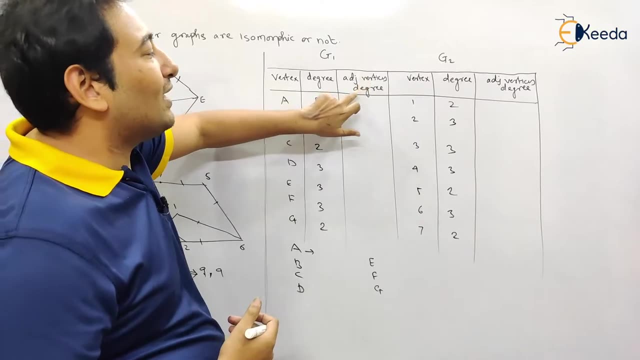 I need to be sure about it, See. So first of all, there is an extra thing that we need to do here. First of all, let us find it out, Then we can conclude. Adjacent vertices: degree. What do you mean by that? 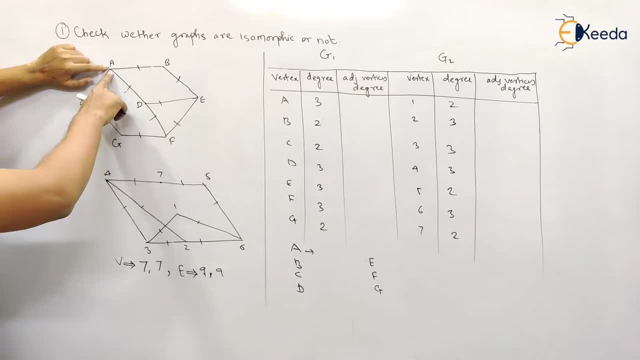 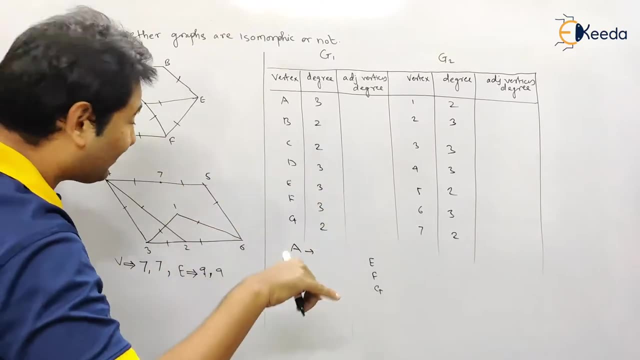 See here: This is your A. A degree is 3. And it's adjacent vertices degree. we need to find it out. This is your Point number 4 that we haven't discussed in detail in video number 1 that we are discussing here. 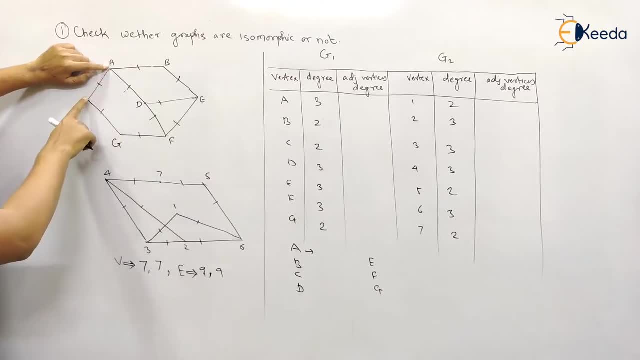 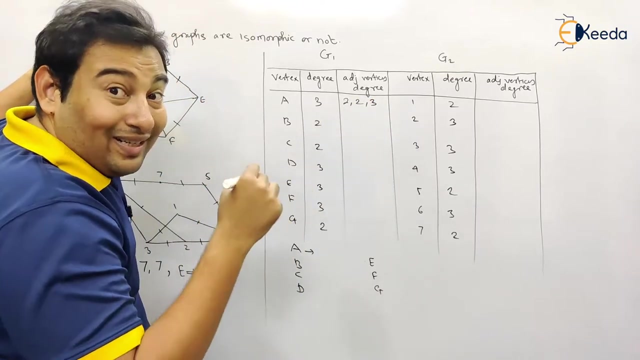 A has 3 degree and it is connected to C, which has degree 2.. A is connected to B, which is again has degree 2.. And A is connected to D, which has degree 3.. So we need to write it down: the degrees of adjacent vertices. 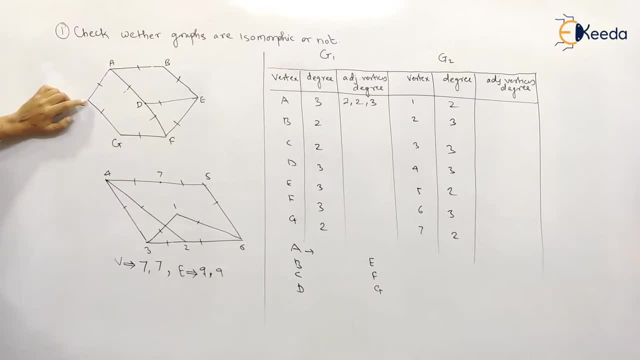 C Adjacent vertices means that is connected. C From C. It is connected to A, It's degree 3.. It's degree 2.. So 3 and 2.. Next, From G From C. we found out Right. 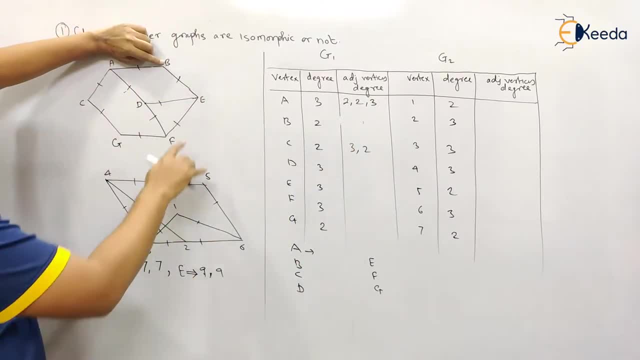 3 and 2.. Let's talk about B. Where is B? B, 3., 3.. So there are 2 connections: Each adjacent degree 3, 3.. Next D: 3., 3 and 3.. 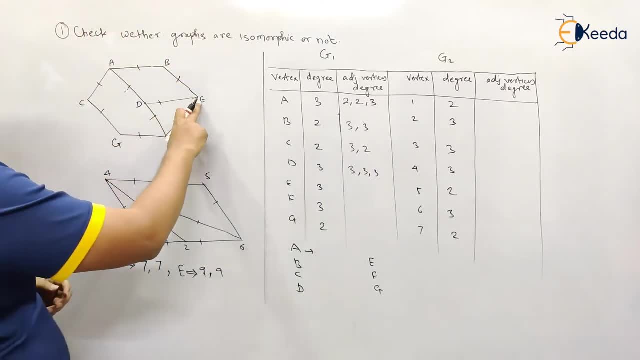 Next E: E 3, 3 and 2.. Next F: 3, 3 and 2.. Next F: 3, 3 and 2.. Next G: Let's check about G. 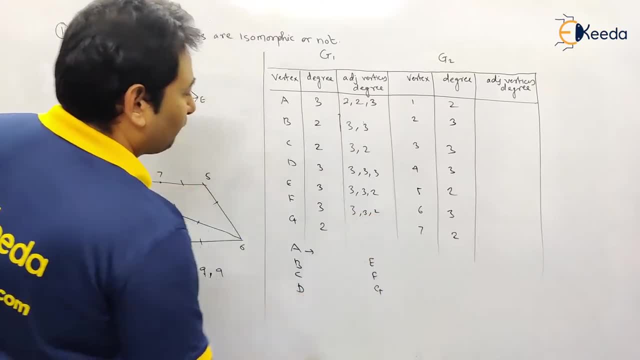 Let's check for G 3. 2.. Let's repeat the same procedure for graph number 2. 1. The connected vertex is 3. That's 3. 2.. Let's repeat the same procedure for graph number 2.. 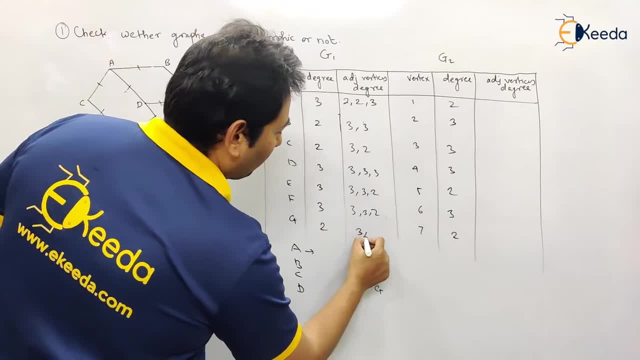 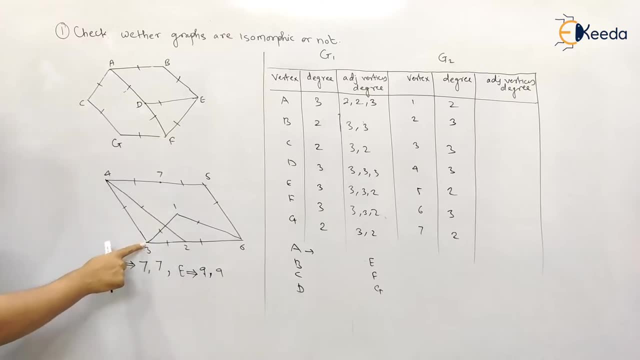 1. The connected vertex is 3.. That's 3., 2., 3., 3., 2., 3., 3., 3., 3., 3., 2., 2.. Next 4.: 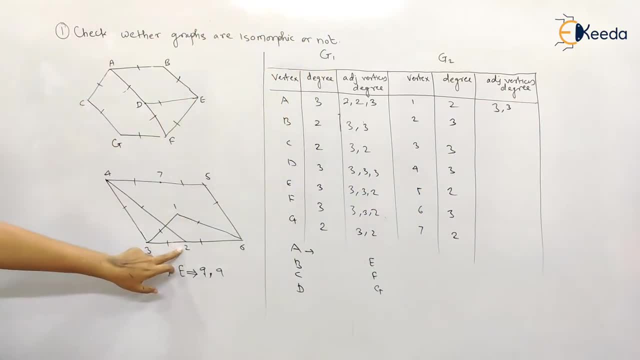 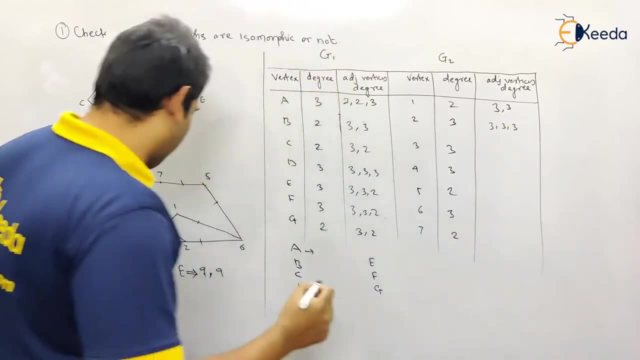 2., 3., 3. Next. 4. 3., 3. 3. Next. 4. 2., 1., 3. 1., 1. 1., 2., 1. 2.. 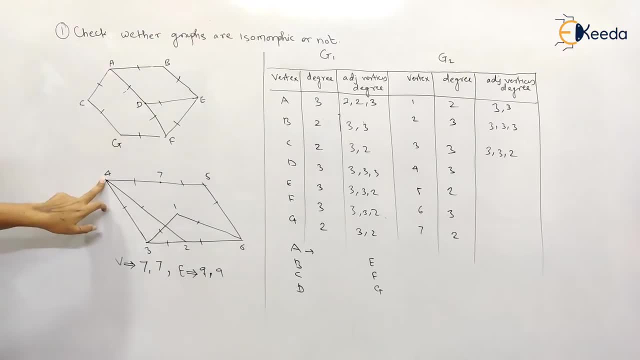 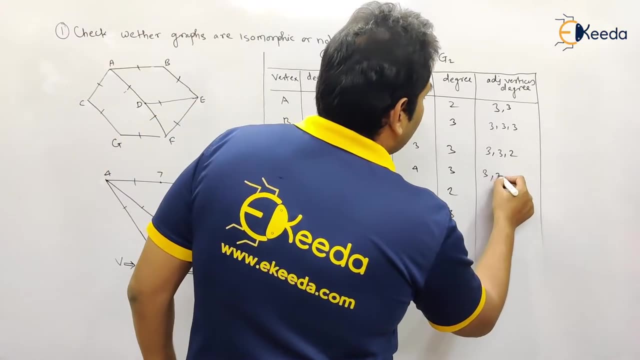 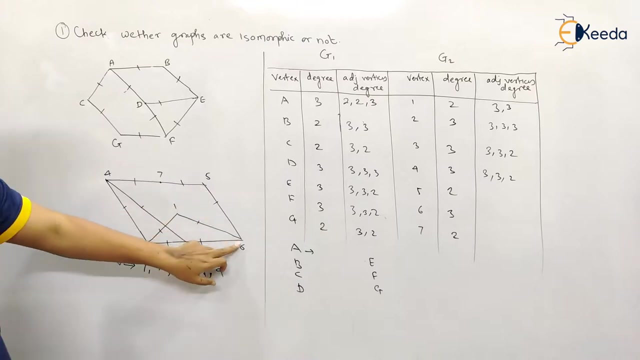 2., 1., 2. 1. 2 by 1., 2 by 2., 2 by 1. again Now Motors of 3.. three, that means three, three, two. basically, are you getting right? next: five, three, two. 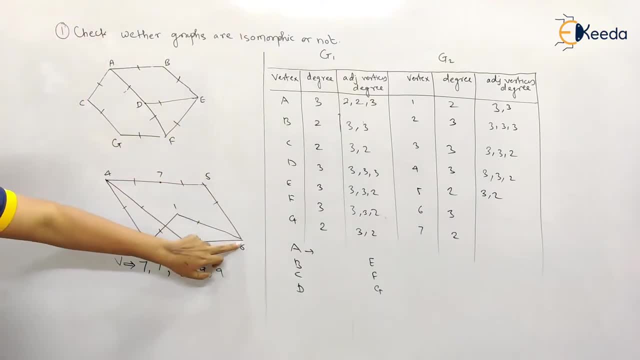 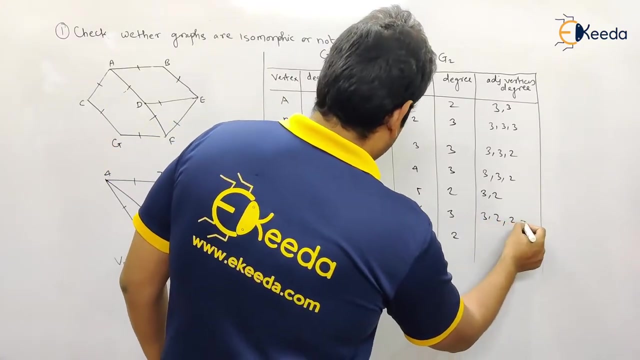 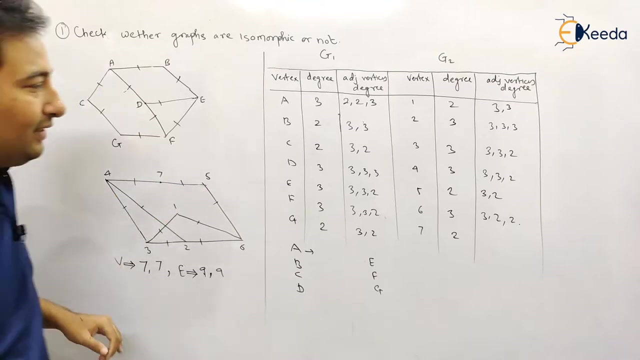 six, two, two. sorry, there is no point here. uh, for six it is two, two and this three. that is three, two, two, seven, next finally seven. for seven, the connect rates are two and three, or you can say three and two, two and three and two, doesn't matter. 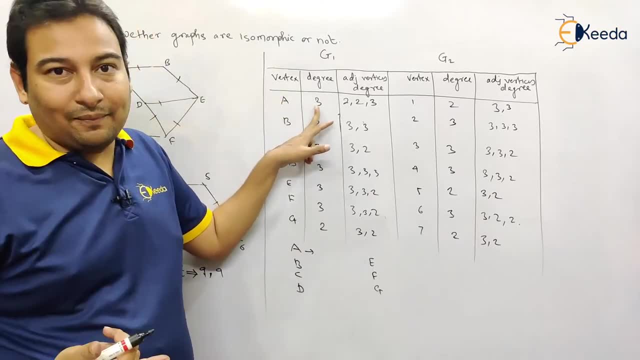 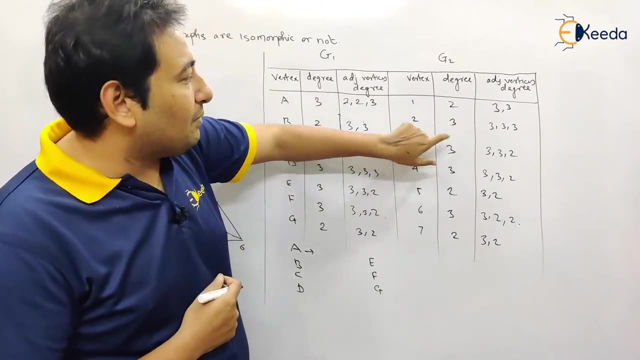 now. we then need to rename it a. what are the options? see: a has degree three. now a can be mapped to what? a can be mapped to degree three? it can be mapped to two, it can be mapped to three, or it can be mapped to four, or it can be mapped to: 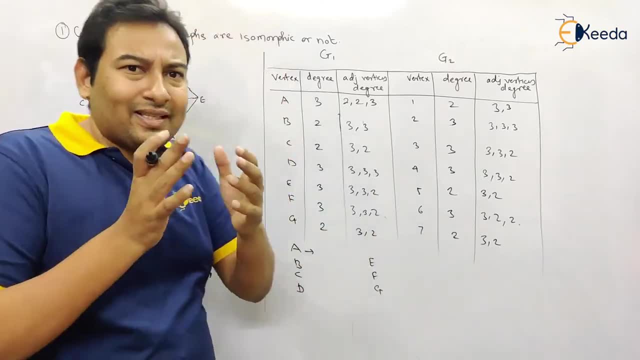 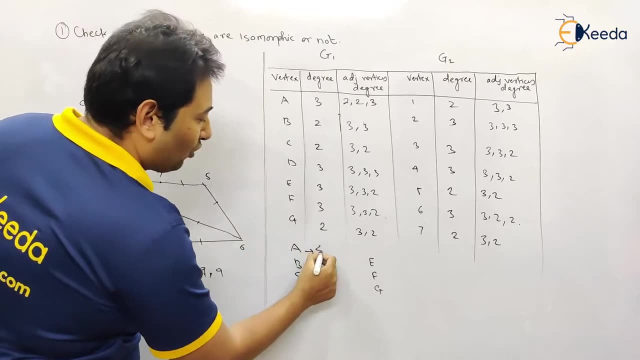 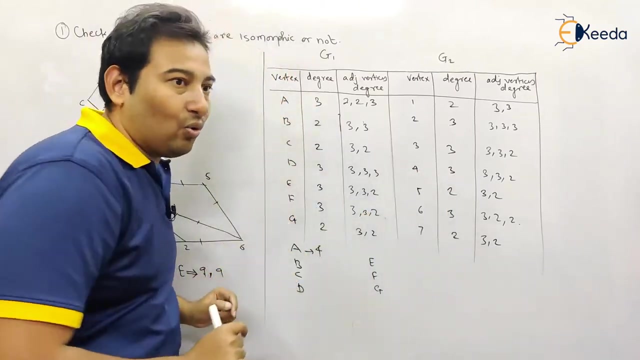 directly blindly mapped it. why we directly blindly mapped it? because every vertex was degree two. but here we cannot map it. that means i cannot map a to four. that is not allowed. now you might be thinking: a degrees four, a degrees three, four degrees, also three. so it should be allowed. 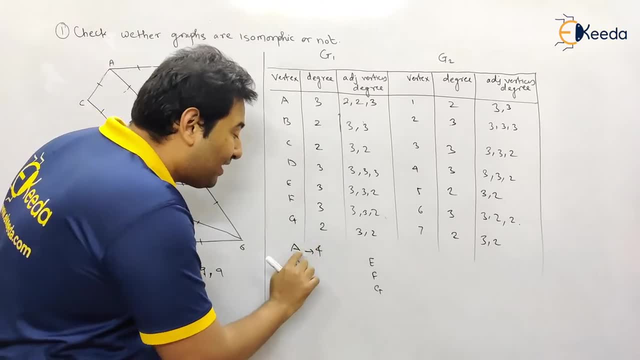 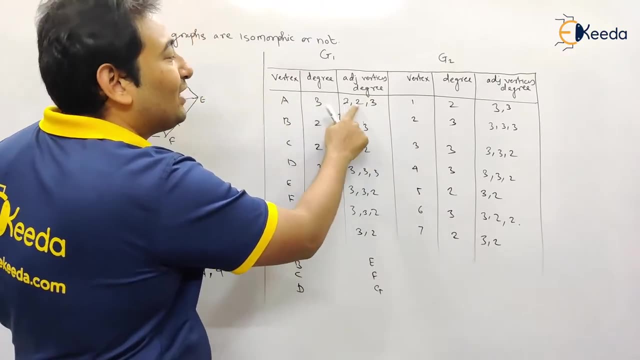 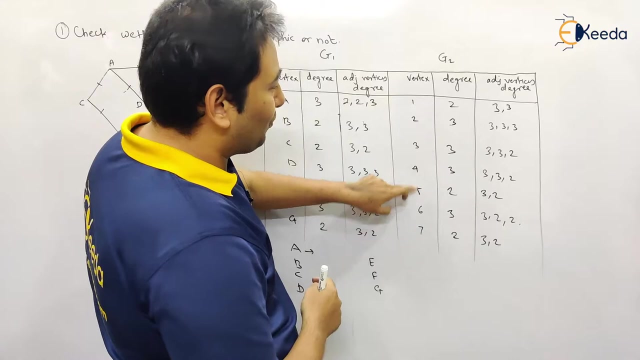 no, this is not the concept of adjacency. adjacency means see the a adjacent vertices has degree two to three. so i need to check these two conditions, both condition we need to check a degree has three. so i have now one, two, three, four options out of four options which adjacency? 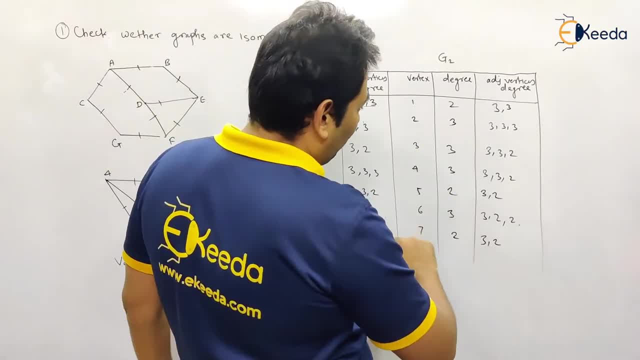 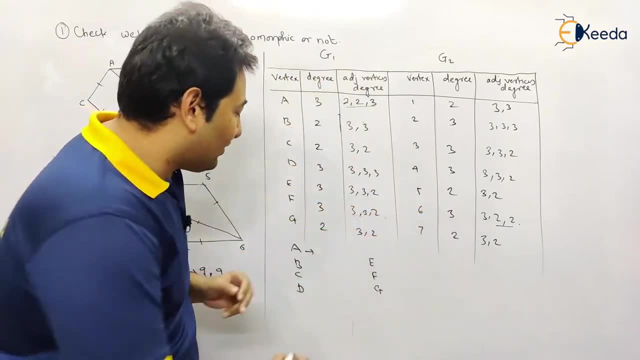 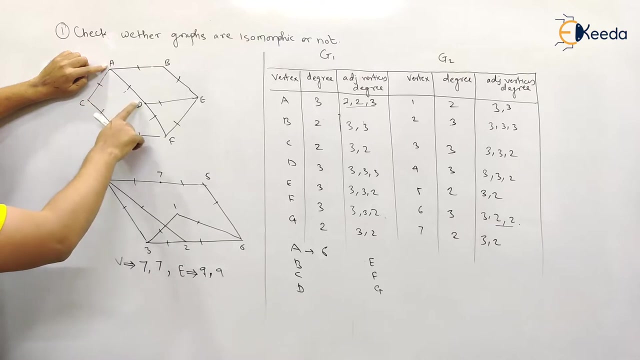 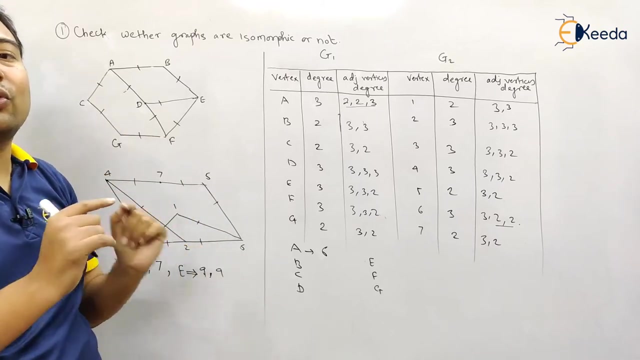 is two to three. that i need to check. so two to three, see here. two to three, that means a can be mapped to six. now let us check, see, a can be mapped to six. both have degree three and it's adjacent degree two, two, three, two, six, adjacent two, three and two. so both the condition must be satisfied, then only. 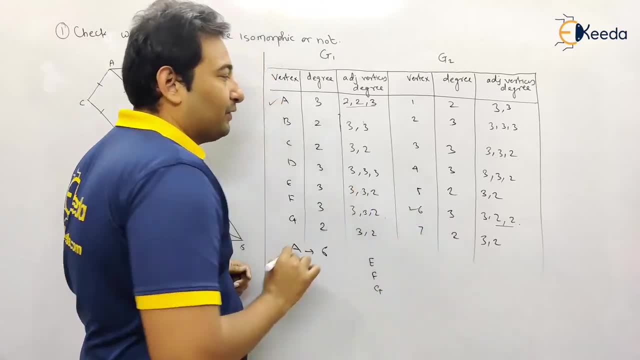 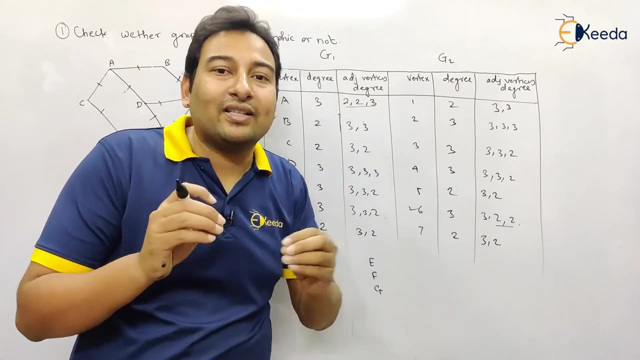 you can map it. so a and six are done. are you clear? so this was the difference between the last problem and this problem, because in the previous problem every vertex and adjacent vertices, degree were two, because everywhere it was two. so the fourth point was not discussed in. 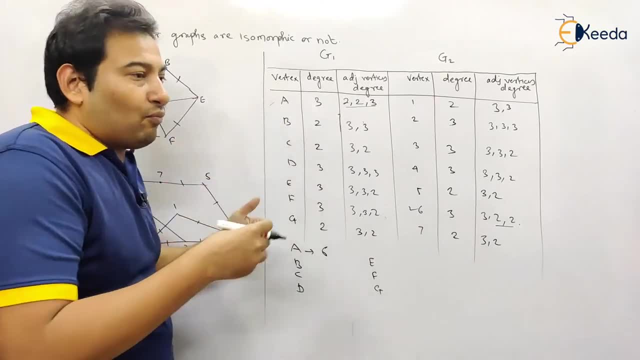 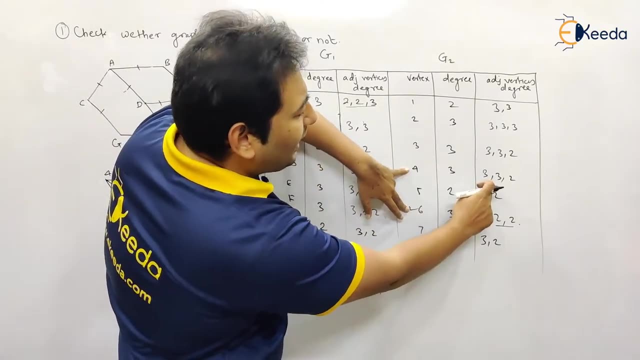 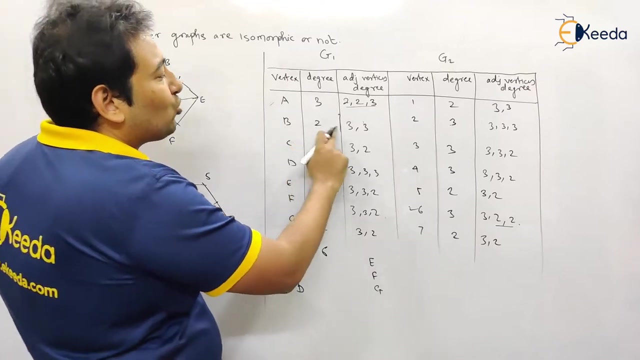 detail, let's move on. let's talk about b now. if there are more than one possibilities like six and suppose, suppose four, also the same condition satisfying both three and two to three, then in that case you can go either, for you can choose any one. let's move on b. so b is two, three, three. so let me check. 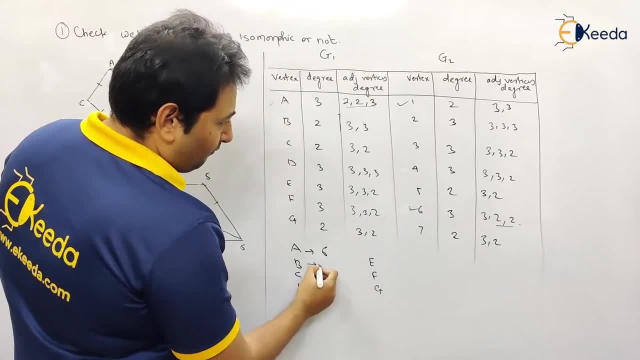 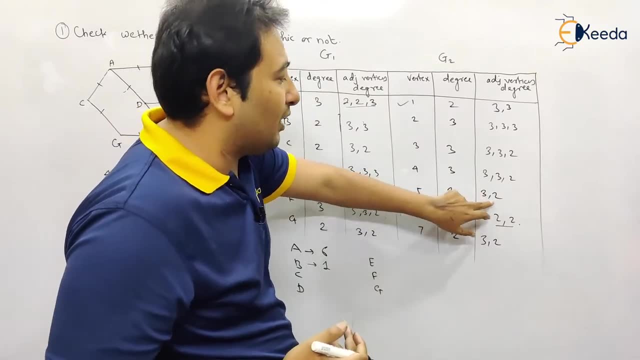 two, three, three. that means you can go ahead with one. next other two option was this: so that is not allowed, because this is three, three and this is three, two, suppose it would be three, three. so that is fine, you can go ahead with one or you can go. 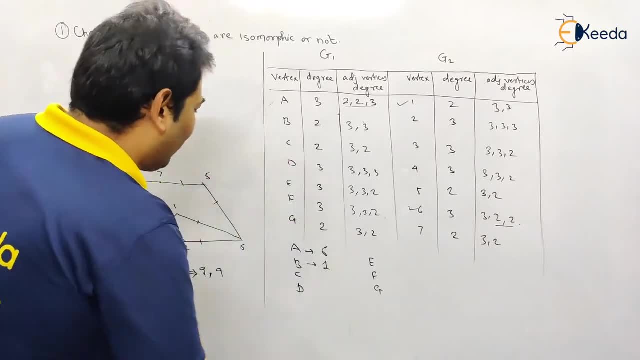 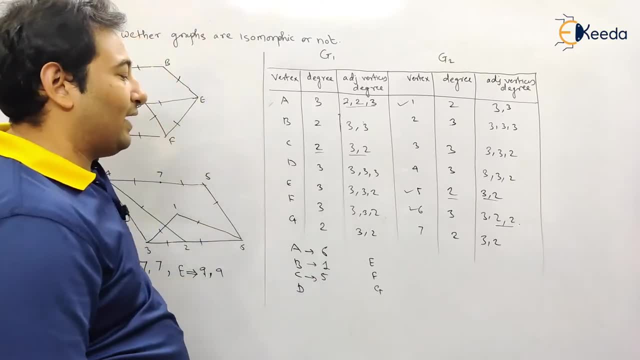 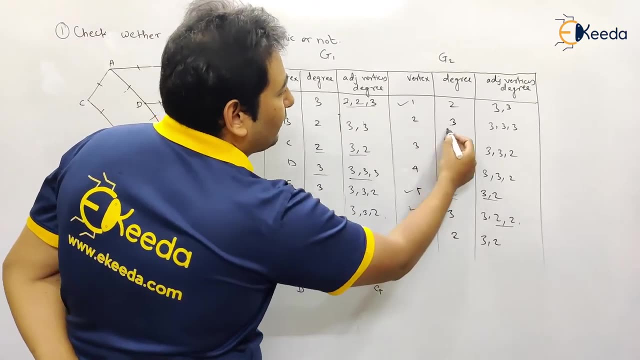 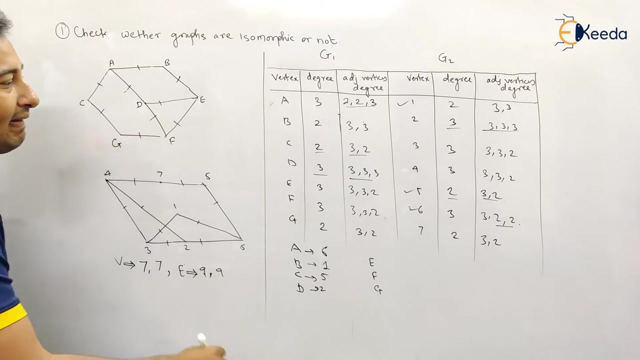 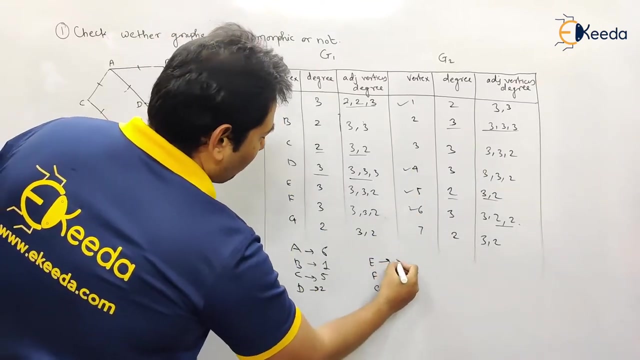 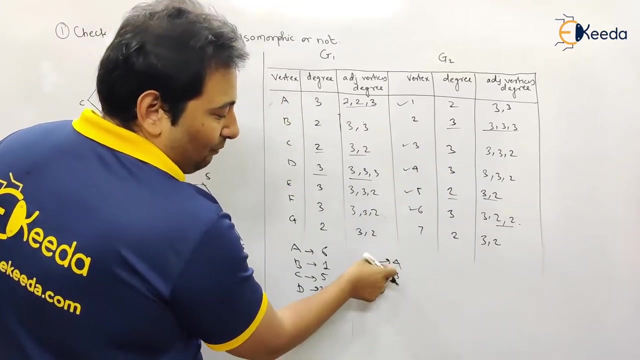 C, it's two, three, two. so two, three, two. still marred to under guide three and triple, three, see that means this is equivalent to two. next you, two. an charge on the current three, three, three, two. that means four, f, three, three, three, two, c, three. obviously you can swap both and g. finally, two, three, two.